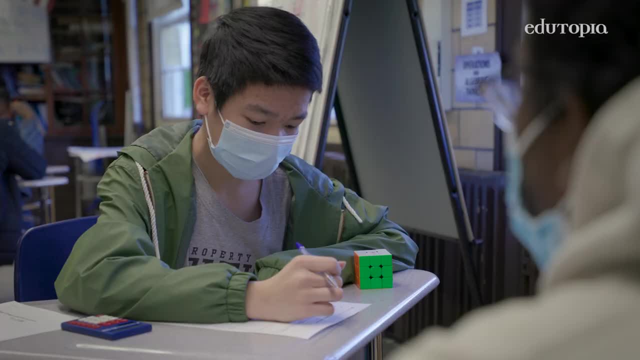 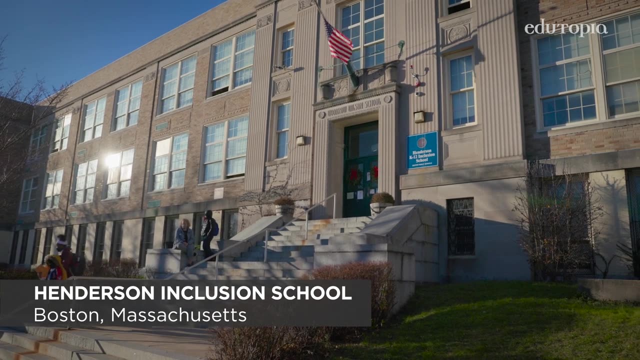 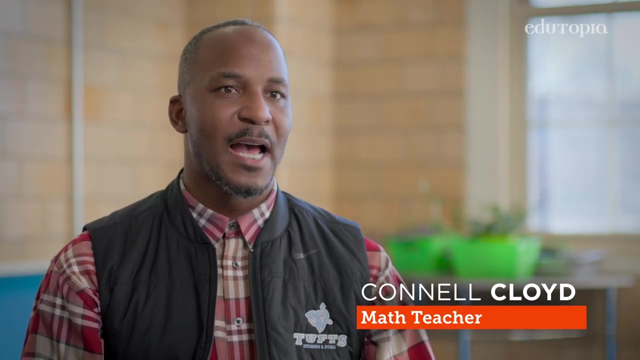 using that questioning language. It really strengthens the discourse between the kids. Good morning everybody. So we're conducting our math interviews today. Before I started, I would get a lot of well, I don't know, I don't know, I don't even know where to start. 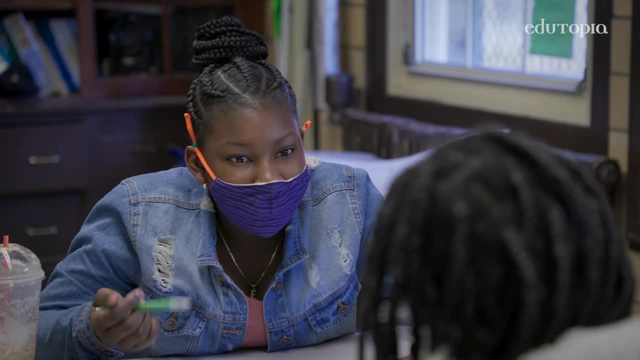 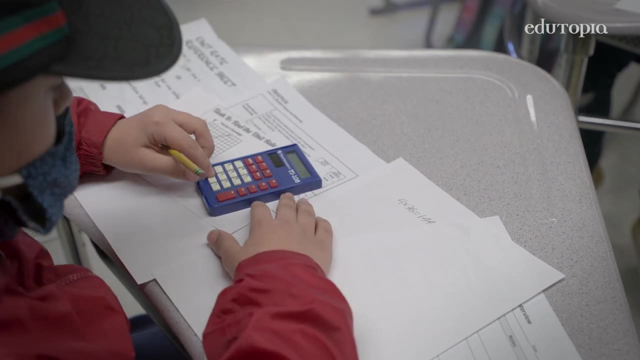 And now, before they call me over, they've either asked a peer look around to check the anchor charts, or they've written down something that they know about the problem. Each of you will be given one task. Either you'll be task A. 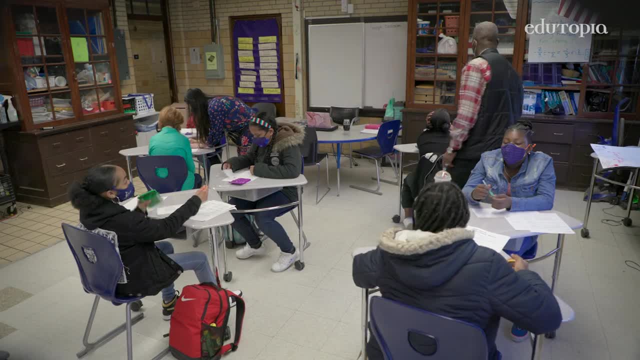 or you'll be task B, First five to seven minutes of collaboration. you'll go through the math interview and then you're asked to do a couple of things. you work on your problem, I work on mine. we cannot help each other at all, but you 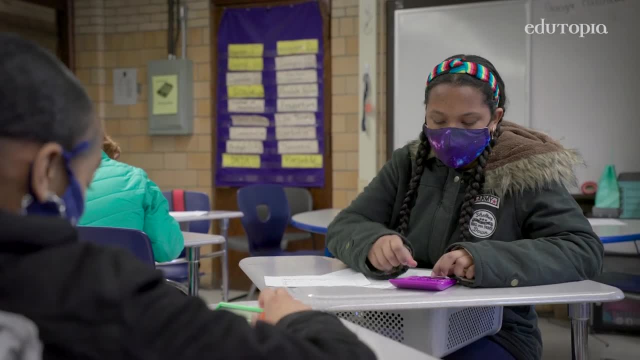 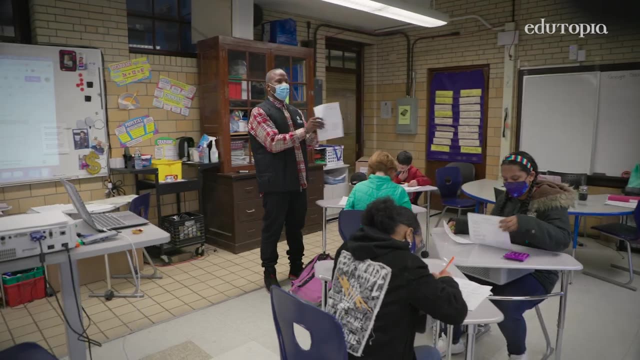 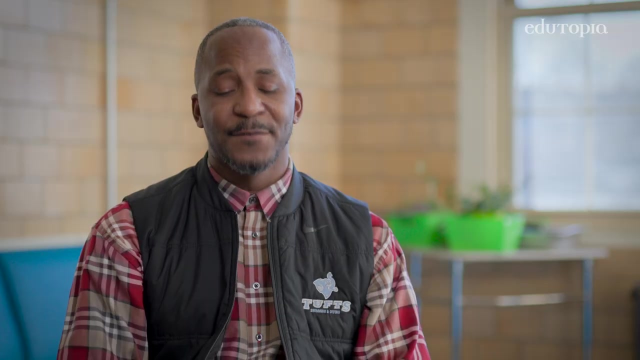 don't have to have the right answer to conduct a math interview. so, task a: write your partner's name on your paper, on the interview paper. everyone has the document with the questions all laid out. with task a, you can begin interviewing task B. now it starts out very scripted. the very first question is when you read: 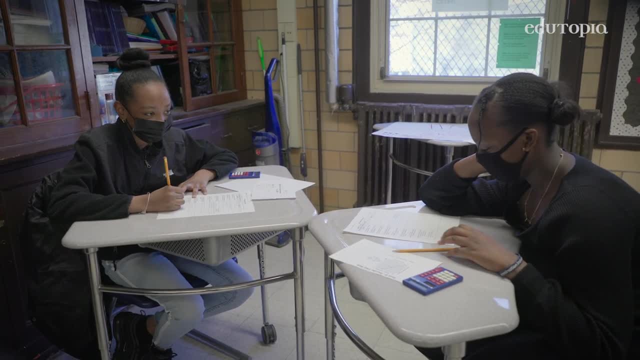 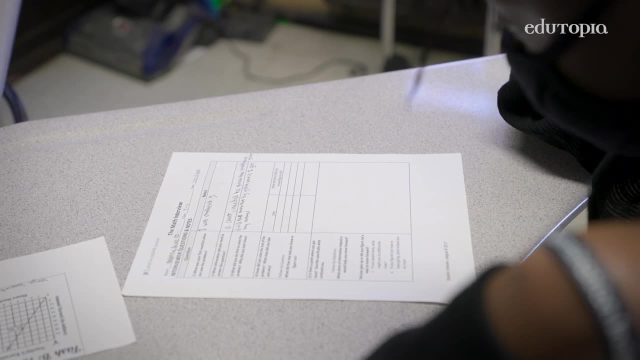 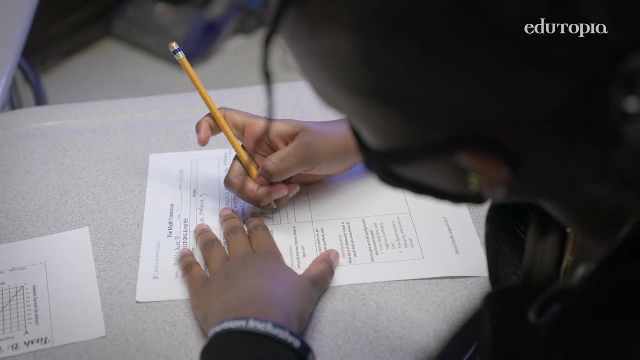 this problem? how did it make you feel that question is rarely asked in math? did you understand what the problem was asking himself and then you get into the nitty-gritty. how did you solve the rest of the problem? what steps did you take and why I had to do line? 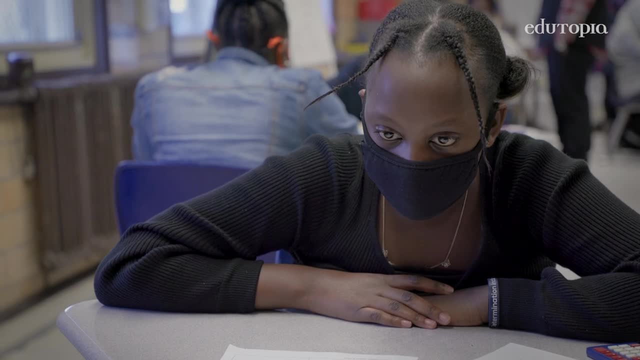 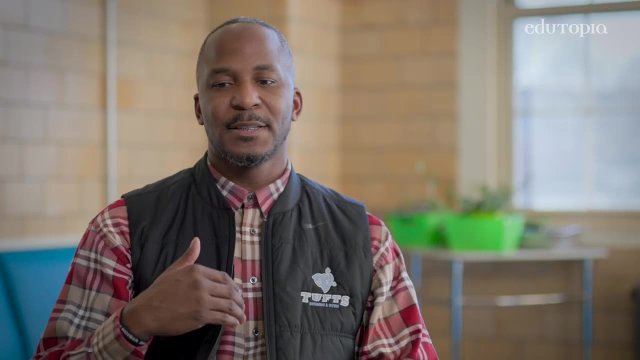 equal sign method, and so now the kids can enumerate the things that they did, and then I had to divide. once you get all of those out, you get more into the like: okay, let's. let's get into reflective questions. okay, have you ever seen a problem like that? 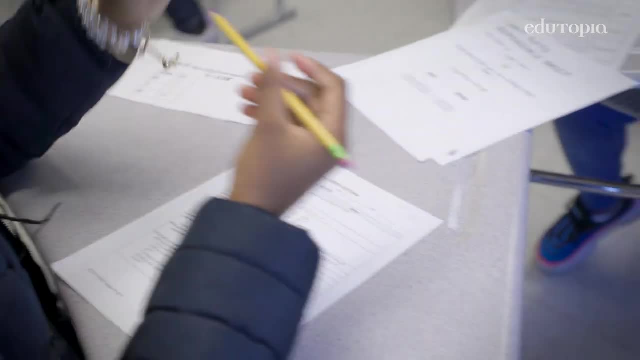 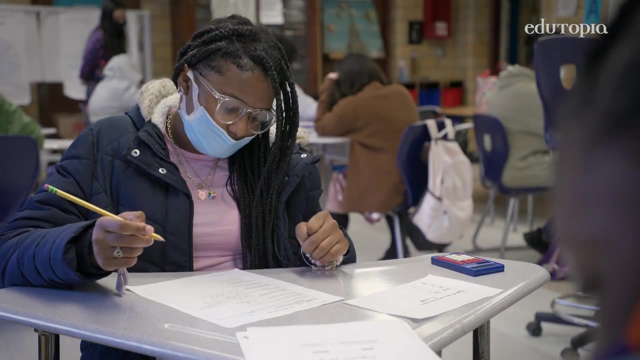 like this before. um, there was a point where I didn't know if the floor goes over the 36 or 36 goes over the floor. did you give up or did you figure out a way to move forward? um, I'm figured out a way to move forward. you can go ahead and. 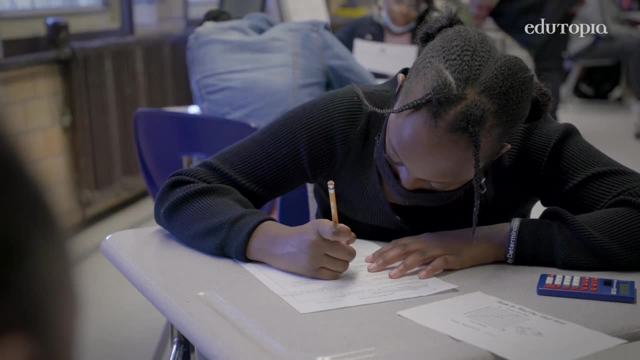 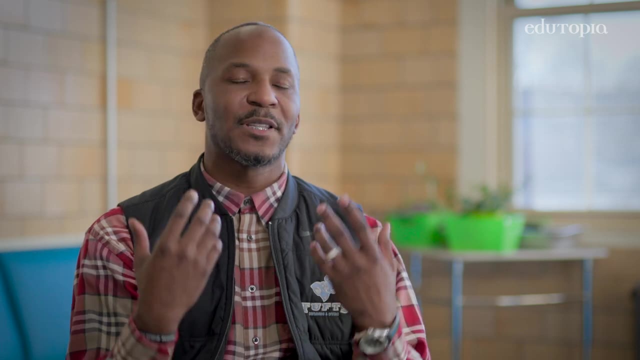 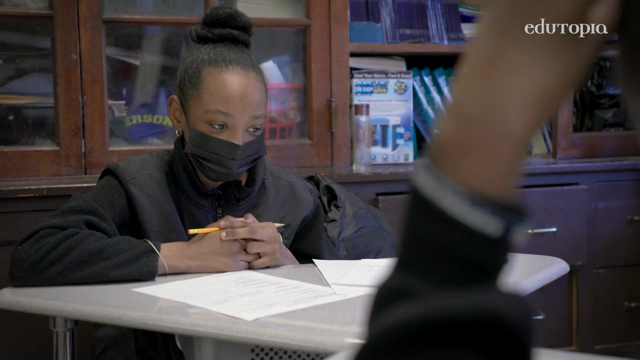 switch. if you have already finished the first interview, after you interview me. if I didn't finish my problem, you can now help me, but only after the interview, because you want the thoughts to come out as pure as possible. what does that help? help you know or figure out? um one thing, I'm really